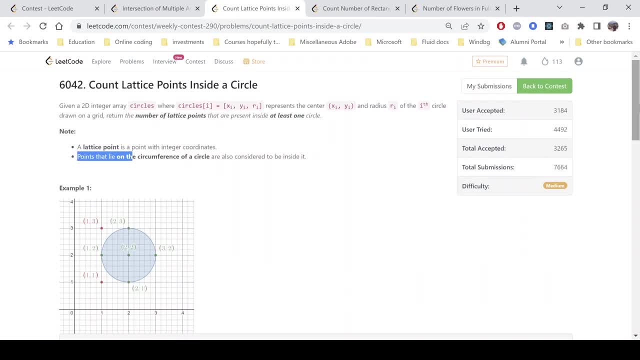 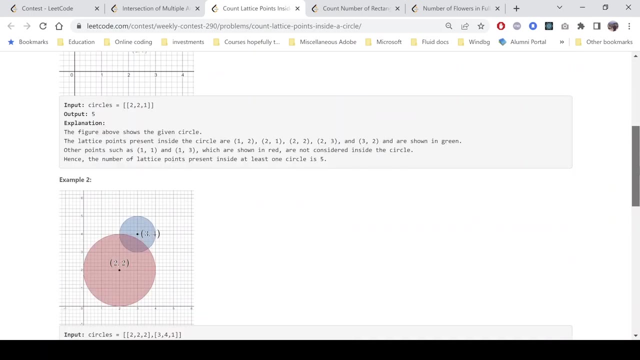 So that means: if you see what a circle is, that means all the points which are present inside the circle and on the circumference of the circle. those integer coordinates will be known as the lattice points. So let's see this one. So we just have one circle. in this case It's 2 to 1. That 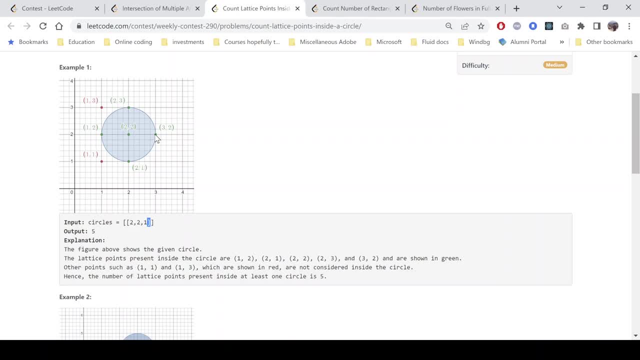 means the circle centered at coordinates 2,2 with a radius 1.. So this is the circle, the highlighted points that we have as lattice points. So if we come from the left, then 1,2 is one of the points. 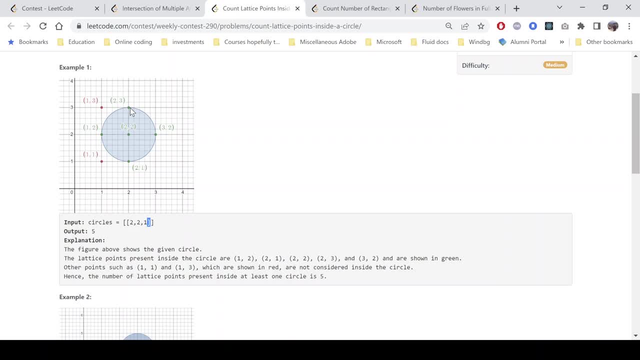 Then what could be the next one? If we see for x equals to 2, that means the coordinate, the coordinates. having the x coordinates as 2, we have 2,3,, 2,2 and 2,1.. So one point was this one: 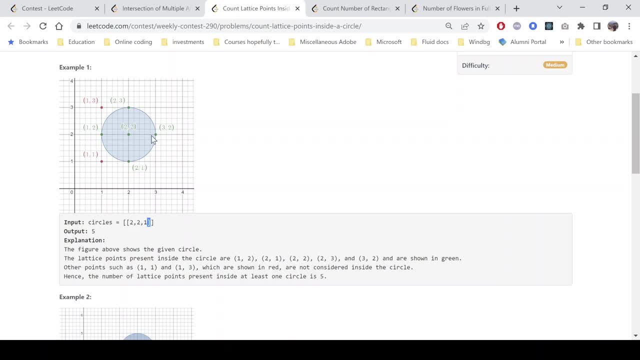 The second is this: When we come to the coordinates which have x coordinate as 3, we have one option. So total we have five options: One when we have x coordinate as 1, three options when we have x coordinate as 2, and one option when we have the x coordinate as 3.. 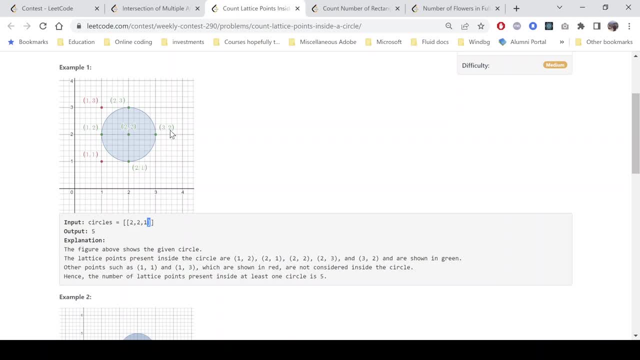 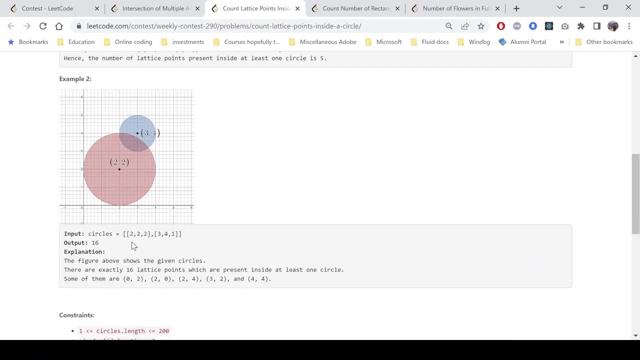 Now we don't need to go beyond this, because those points will lie outside the circle and those will not be the lattice points. Similar, we can see example number 2.. In this case, again, we are given two circles. One is, this is 2,2 and the radius is 2 again. 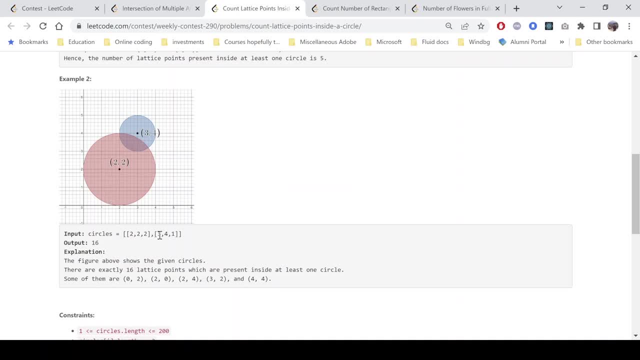 So the orange, one orange or red, whatever you say it. The second circle is 3,4 with a radius of 1.. So these are the two circles And again, if we move from left to right, these are the points. 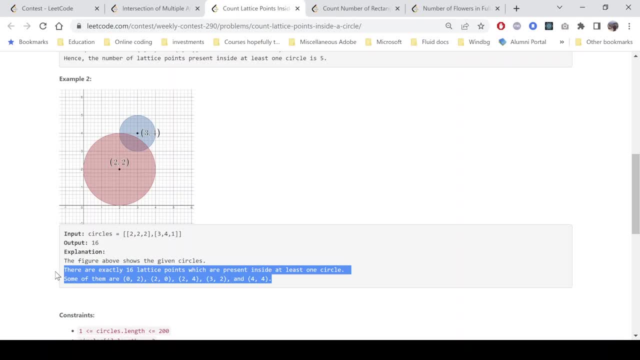 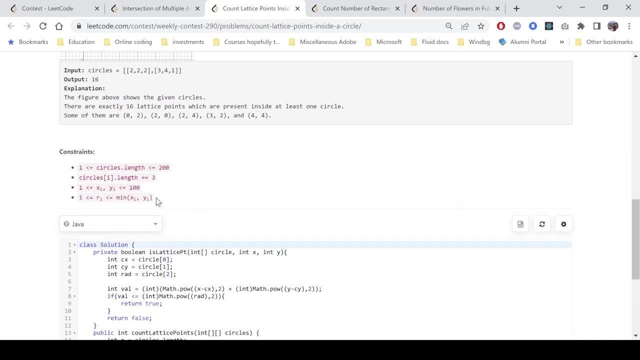 that tell that these are some of the lattice points, So we'll see how we need to compute it. If we come down these constraints will be very helpful for us in devising the algorithm. So it says that the number of circles that will be given will be: 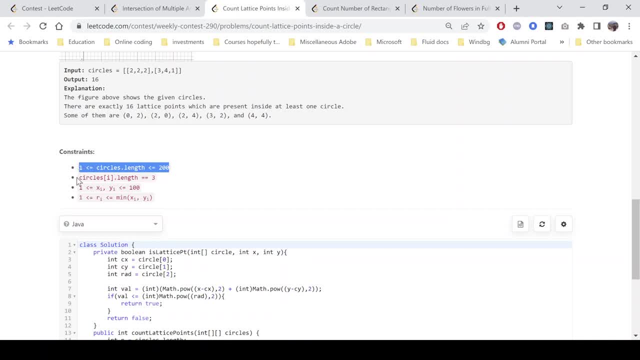 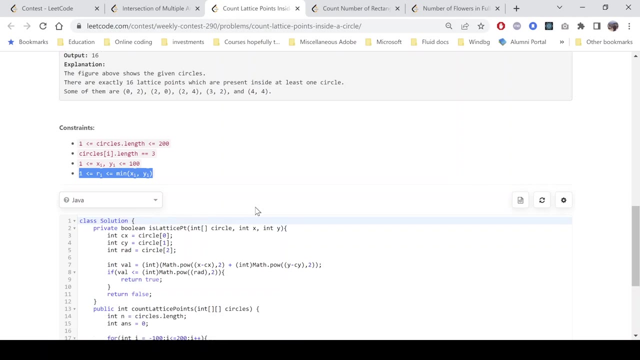 200, like the max number of circles will be 200. The length of each circle array will be again 3. The coordinates will lie between 1 to 100. And again radius will be minimum of x coordinate and y coordinate of a circle. So that means if I consider then my radius, or I would say 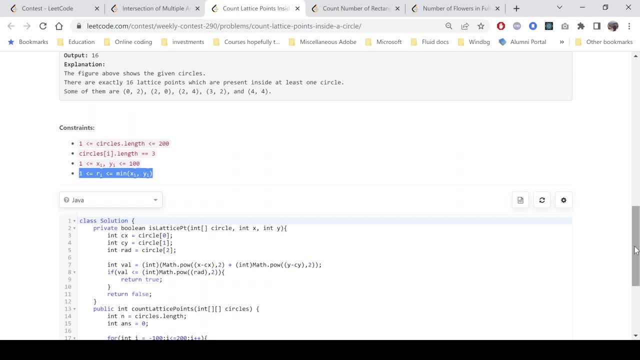 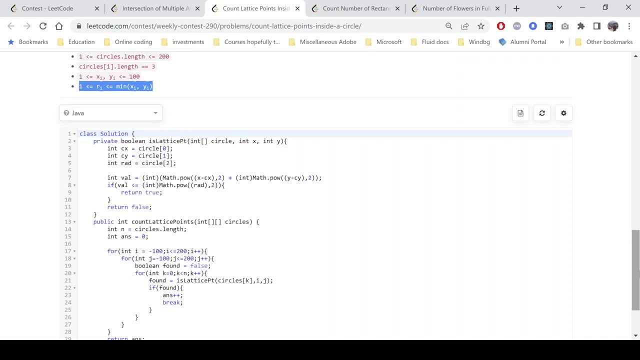 the leftmost point, in worst case, can lie between minus 100. Because if our coordinates is 1 comma 1 or 1 comma 100, whatever it is, and if we and if the radius is, though it says, minimum of x comma x, i, comma y, i, But again, if you consider the maximum value of 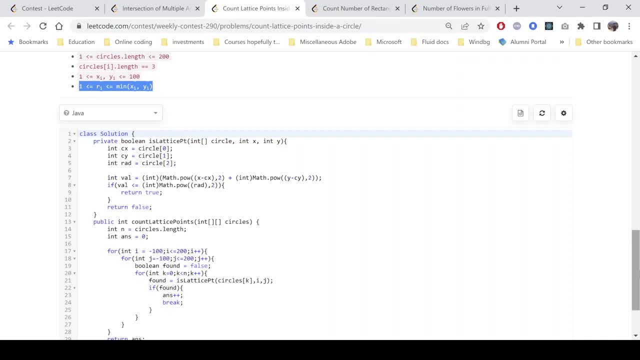 the radius, that will be 100. So it will be minus 99.. And if I talk about the rightmost extreme, that means if our x and y coordinates is 100 comma 100. And in that case radius is also 100, as the question says. So 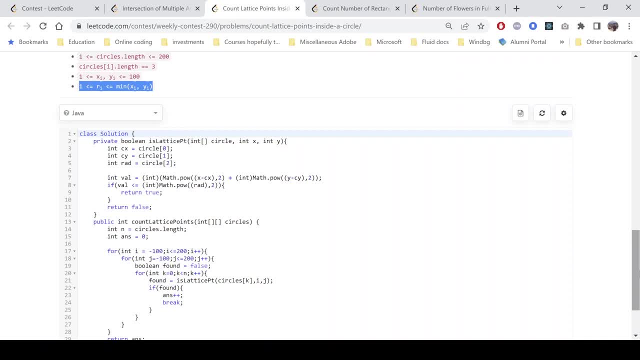 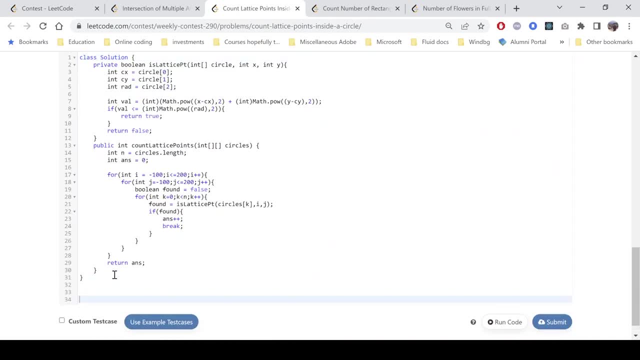 that will the, the, the x coordinate will go maximum up to x and y coordinate will go maximum up to 200.. So if I explain you by writing it then you can see that it's one comma. the x and the x and y lie between 1 to 100, 1 to 100.. I'm writing on line number 34, 1 to 100. So that means, even if I 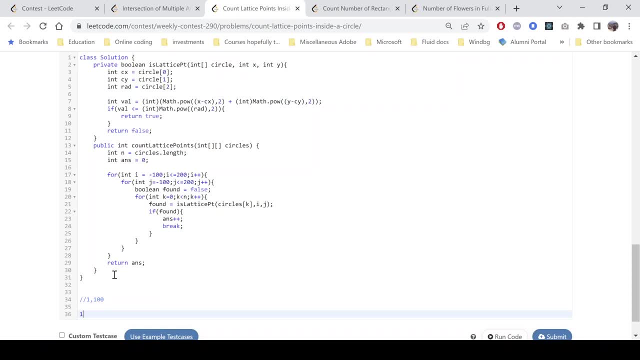 consider the radius of the radius to be 100, then what would be the leftmost coordinate? The rightmost coordinate would be 1 minus 100, comma. what could be the rightmost coordinate Again, if it is 100 comma 100, so it will be 100 plus 100, that comes out to be 200.. So we are doing. 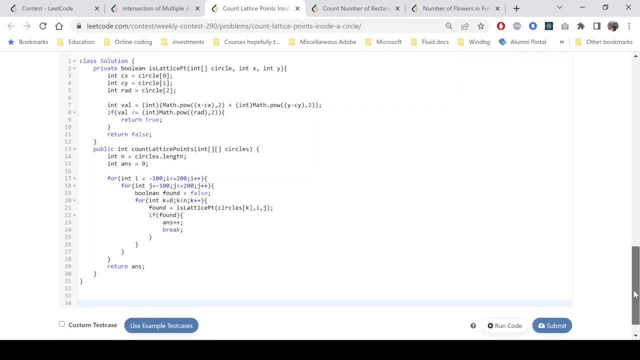 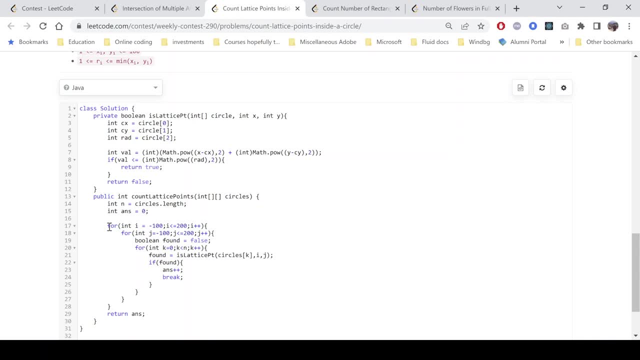 a brute force here, because the constraints are pretty low. So all we need to do is we need to run a loop from minus 100 to 100. So we are running a nested loop. The first one is for the x coordinate. what are the possible values of the x coordinate? The second one is: what are the 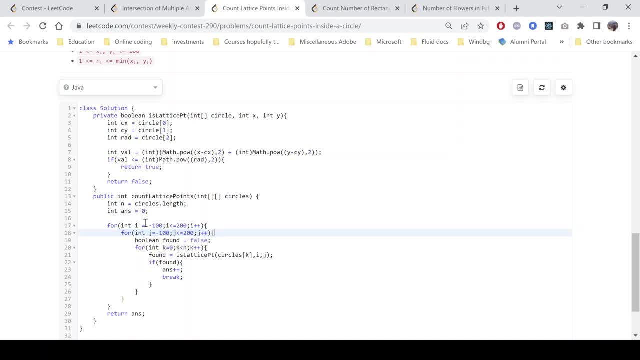 possible values of y coordinate. Okay, And so again, as we saw in the explanation, it could go from minus 100 to 2 plus 200.. Again, it should go from minus 99, but again I've taken it minus 100.. 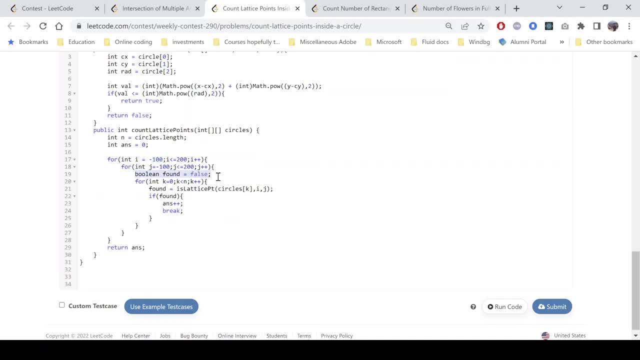 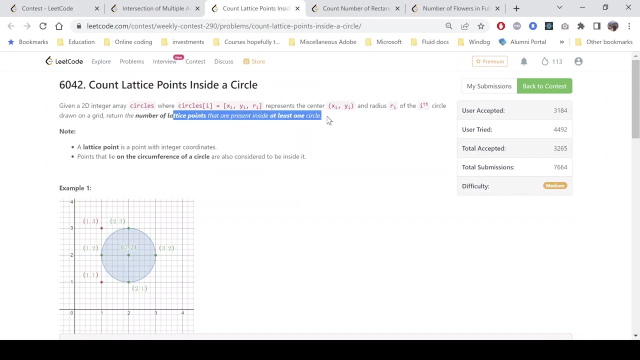 Now we have taken a variable that whether we have found a lattice point or not- we'll see why I've taken it- And then we traverse the number of circles that we are given. Now if you see in the number of lattice point that are present inside at least one circle, that means as soon as we find. 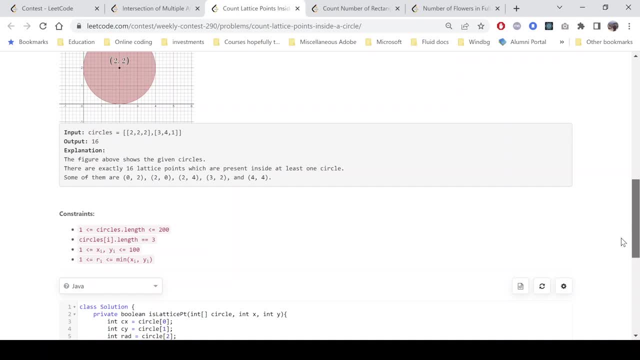 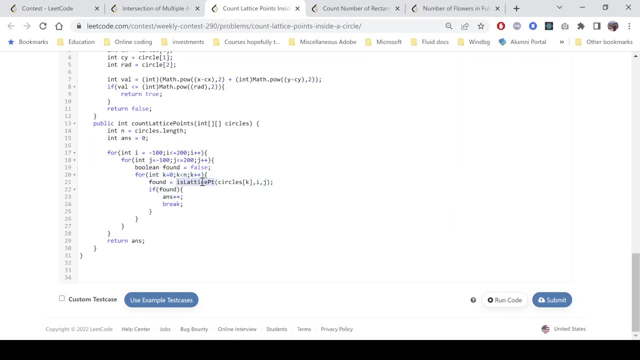 that a point is present inside any of the circles, we are good to go. we can add that to the answer. So that means we traverse the number of circles. we call a function that, whether the current point is a lattice point for the current circle or not, the current circle is the kth circle. 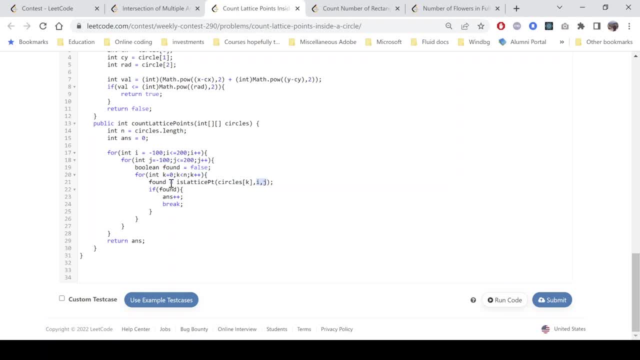 we pass the x and y coordinate, that is, i and j, And if we find that the current is a lattice point, so we increment our answer. we break the loop because we don't need to traverse for the other circles for this coordinate because this already is a lattice point, so no need to. 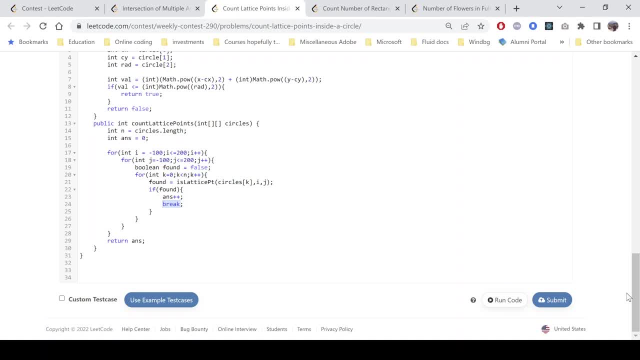 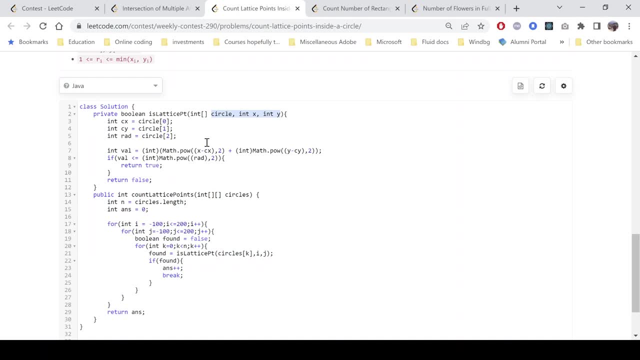 check this point for other circles. so let's see what this function says. this function receives a circle and an x and y coordinate, that is, an i and j from line number 17 and 18. uh, this is just for readability. i've done now, uh, for a circle. the formula of a circle is that it, it goes something. 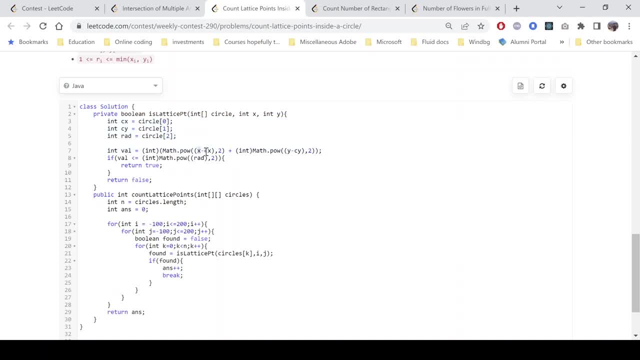 like: uh the x coordinate, uh, so you can just reverse it, but again that would work. so it says that, uh, the point that you have received, uh the coordinate x coordinate minus the center of the circle square plus y coordinate minus the center of the y coordinate of the center of the circle. 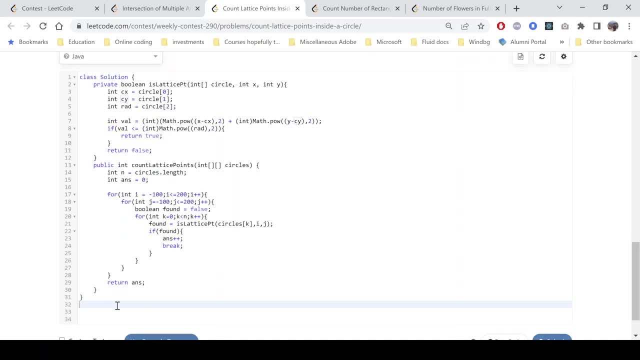 square and that should be less than equal to rate the square of radius of the circle. so if i write it, it would be something like x minus x1, suppose. uh, if i take square, this is the formula. if i write plus, this is: this is right. 2 equals to, again, radius of the circle, r to the power 2. yeah, so this is the. 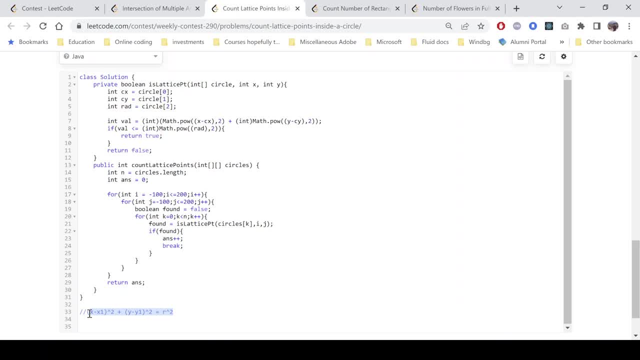 formula of the circle. so, if so, this is the formula of the circle now. if i write it less than less than then, this will represent the all the points which lie inside the circle. now what we need to find: we need to find all the points which lie inside the circle as well as on the circumference, so the formula will become less.